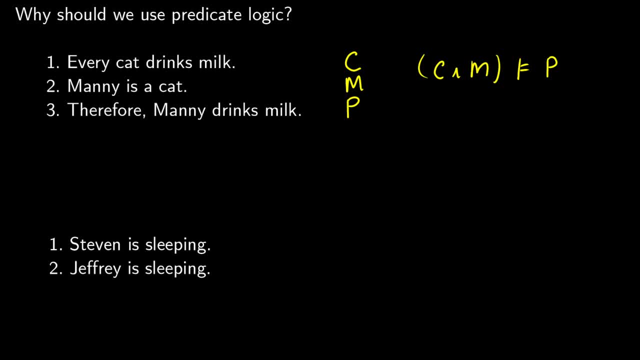 So we could introduce something and say, okay, for all X, if X is a cat, then X drinks milk. We could establish Manny as a cat. So we could say that there's a cat whose name is Manny. Therefore, we have that Manny drinks milk. 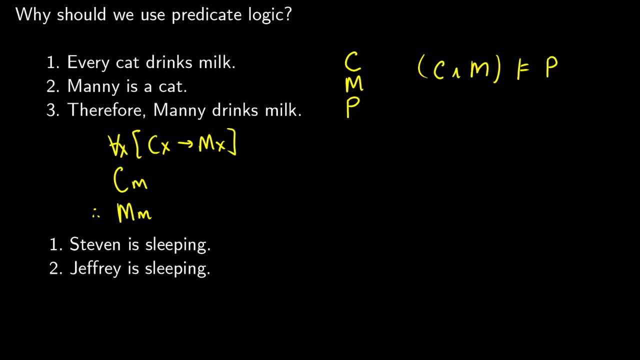 And this notation we're going to learn in this video, but this is just a way that we could symbolize this argument in a way that makes sense. Another reason that we want to do this is if we compare these two sentences, Stephen is sleeping and Jeffrey is sleeping, in propositional logic, we would have to do something like S and J. 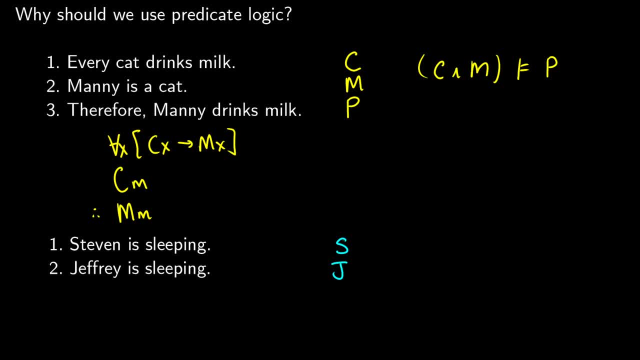 But really, if we take a look at the sentence, there's a lot in common between these two sentences. 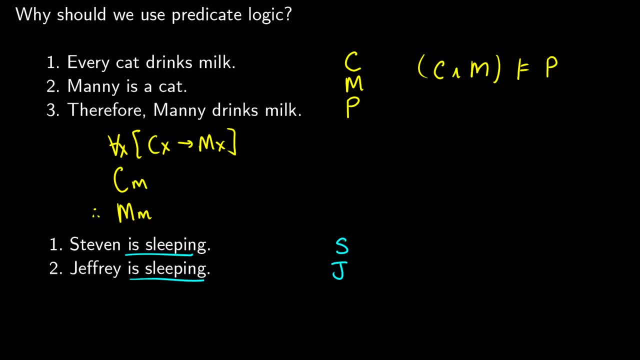 They're both doing the same action. The only thing that's different is that they're both doing the same action. The only thing that's really changing is who is doing that action. 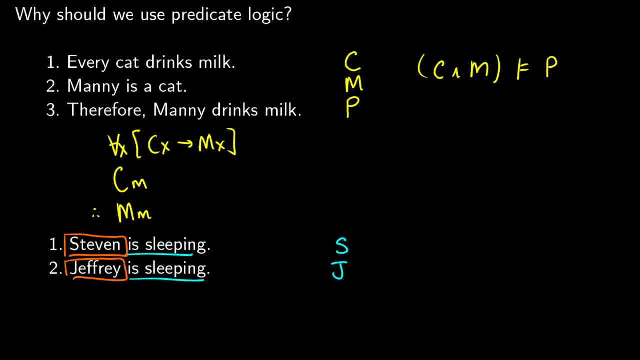 So there should be some sort of connection between them. And with predicate logic, we could establish, say, a predicate like, 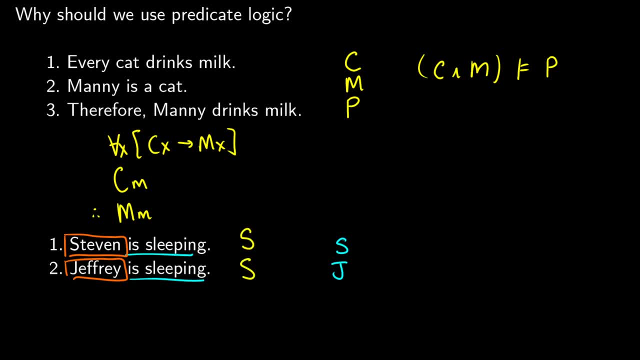 let's say, S means sleeping. And we could pick the little letter beside it to mean who is sleeping. 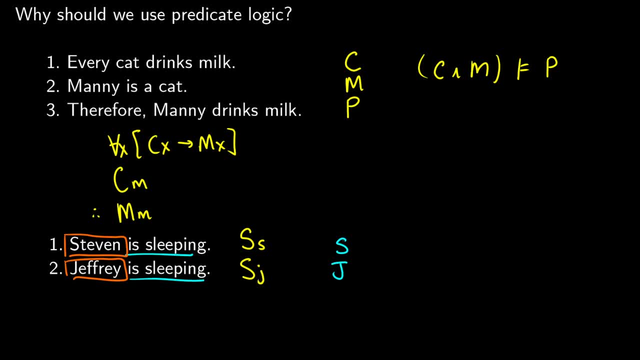 So SS could mean Stephen is sleeping, and SJ could mean Jeffrey is sleeping. And we could make this frame, like X is sleeping. 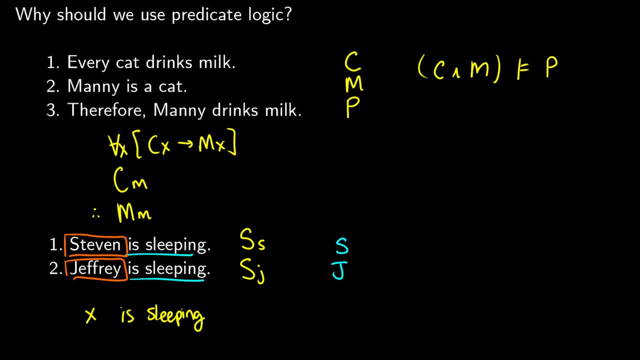 So we could stick in any person's name there. And we could abbreviate this as, say, SX. And then whenever we have someone we want to stick in here, we can just replace it with that X there. 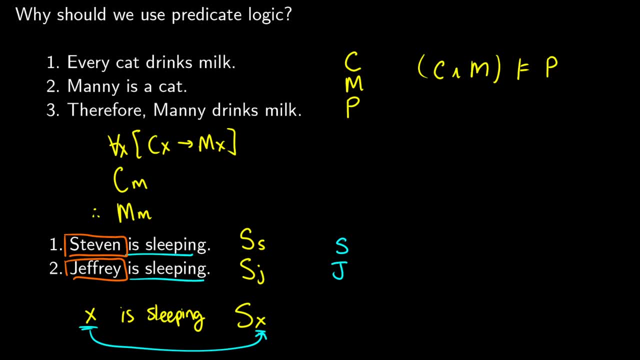 So this is why we want to use predicate logic. So this video is not about translation. 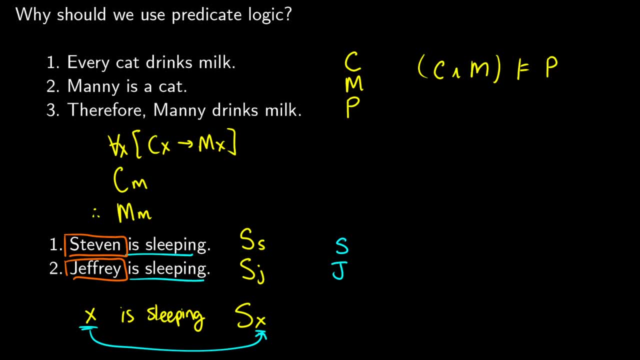 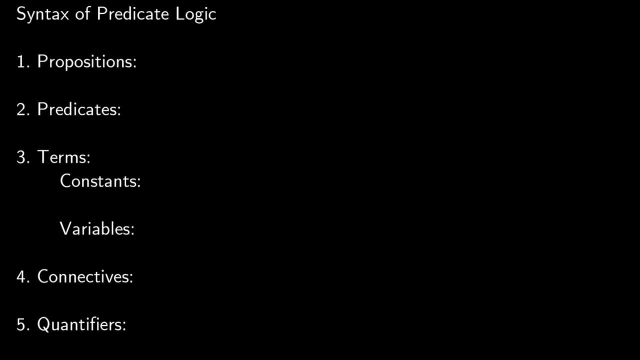 This is just about understanding what all the symbols mean, how we can form well-formed formulas. So the syntax of predicate logic contains everything that we had in propositional logic. So in propositional logic, we had capital letters like P, Q, R, S to mean specific propositions. Well, in predicate logic, we also use P, Q, R, S, and so on for predicates. So we can use these letters. Occasionally, we might also just write out the entire word because it's easier to understand. 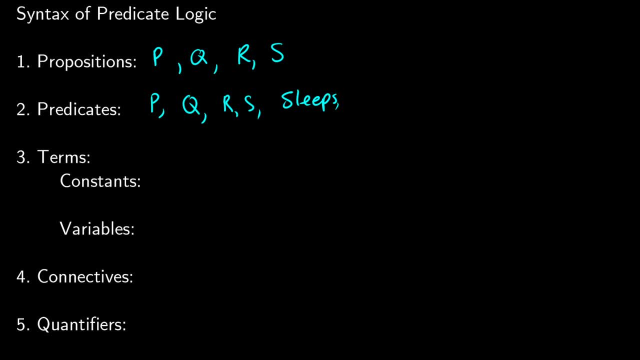 So here we'd say that we have a predicate sleeps, or we have a predicate runs, or we have a predicate dog. So anything that can be given a property, like X is a dog, X runs, X sleeps. You might even have words like likes, or X likes Y. So you can have two things that come after it. Now, predicates are going to combine with things called terms. 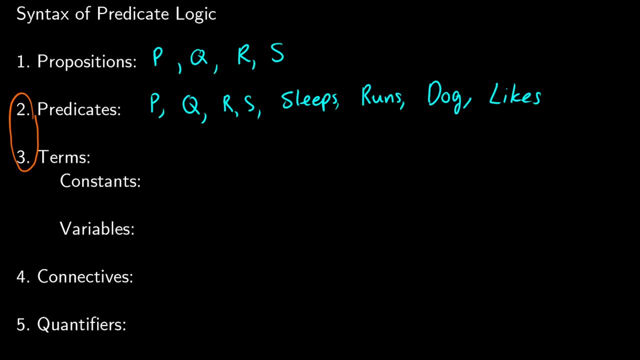 So together, these two create a well-formed formula. And there's two different types of terms. These are our little letters. So we have constants. These are lowercase letters, usually towards the beginning of the alphabet, like J, A, C, B, and so on. And these are usually names of people in our real world, usually what goes in as a constant. 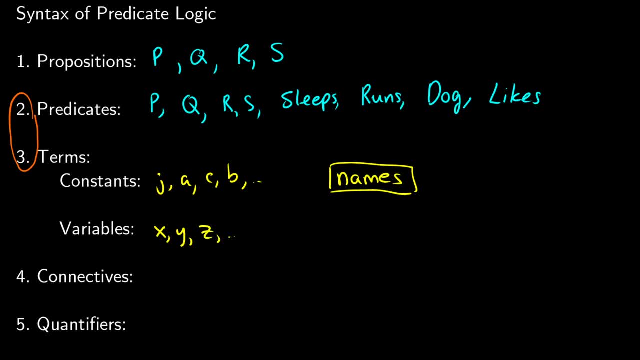 But we also have variables like X, Y, Z, and so on. And these are, of course, our placeholders, or just our variables in general. 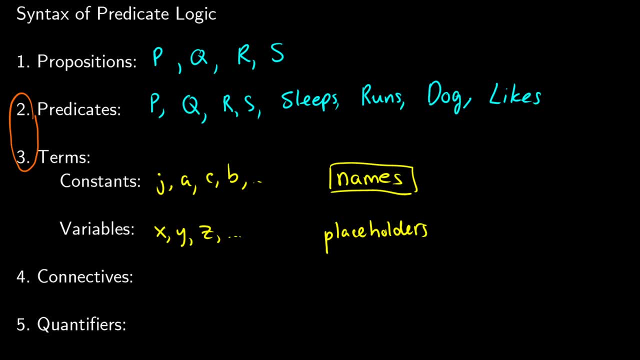 So who is sleeping? X is sleeping. Well, we're going to fill that in with a constant at some point. Who's running? X is running. Well, we'll fill that in with a constant at some point. 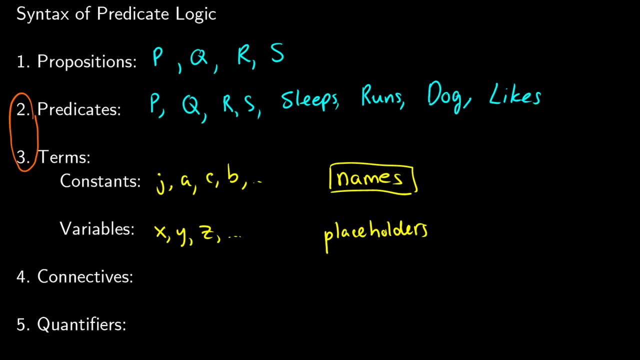 We'll also use variables to combine with quantifiers like all and some in order to give general statements. We have our connectives that we've had before. So we'll have the negation, and, or, the conditional if then, the biconditional if and only if, and, of course, the exclusive or symbol if we choose to use that in our system. And we have quantifiers. 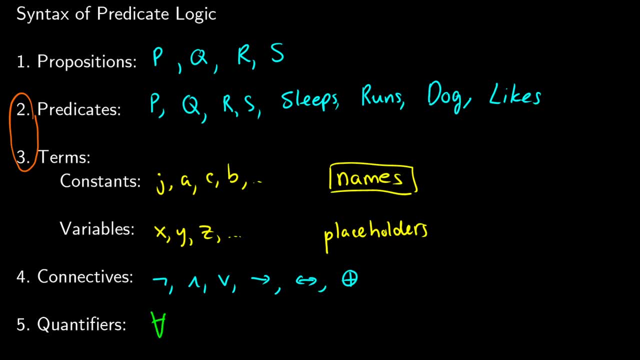 So these are the ones that are probably new at this point. We have an upside-down A, which means all. And we have the backwards E, which stands for existence or existential. So I'll write this down, existential. And this is a word like some. The all quantifier is called the universal quantifier, so let me put this down for completion. So I always remember the upside-down A as all because they both start with the same letter, and the backwards E as exists or a. 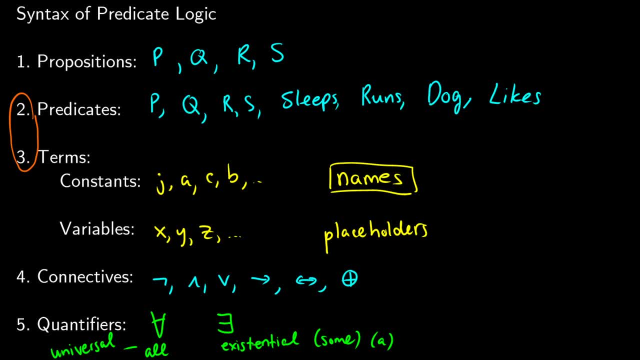 So some is one word to say that, a is another word to express the existential. 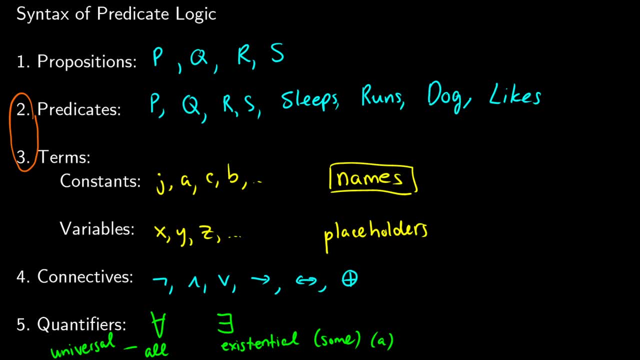 Okay, so with all this information in mind, how do we create a well-formed formula? How do we create a woof? 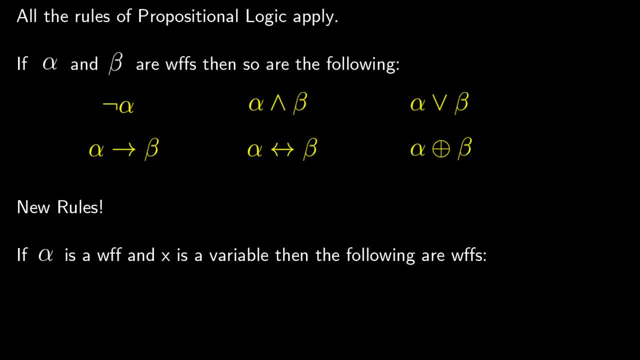 So first of all, if we have any two well-formed formulas, 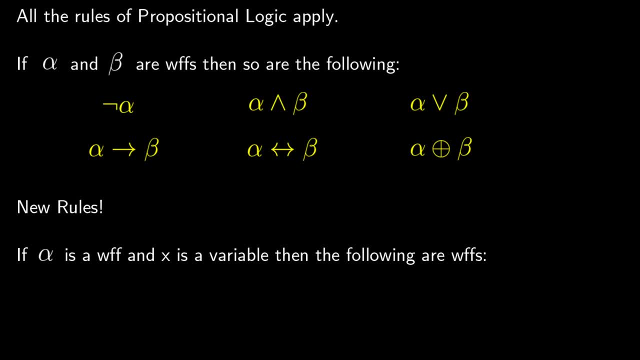 everything from propositional logic applies. So if we have alpha and beta as well-formed formulas, we're going to get not alpha, we're going to get alpha and beta, so we can combine alpha and beta with and, we can do alpha or beta, we can do if alpha then beta, 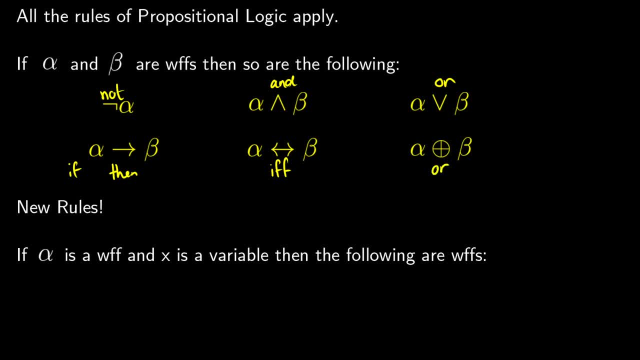 and we can do alpha or beta, but not both. 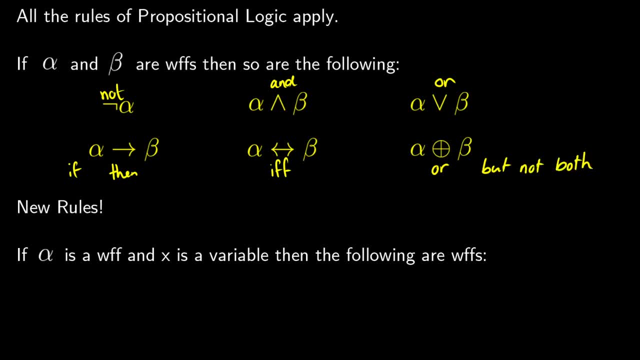 So these are things from propositional logic that you should remember. 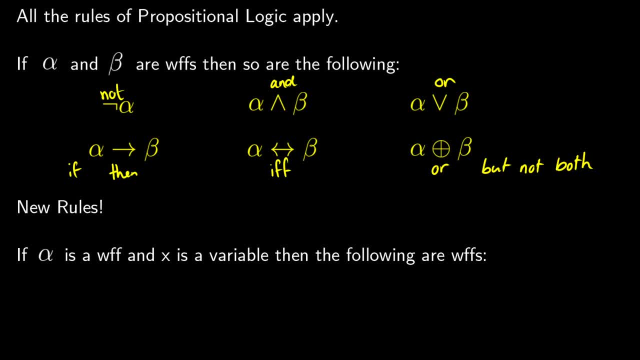 What's more interesting, of course, are the new rules that we have. So if we have any sort of well-formed formula alpha, we can stick a for all x in front of it. So this would be read as for all x alpha, and we'll see how this is used. 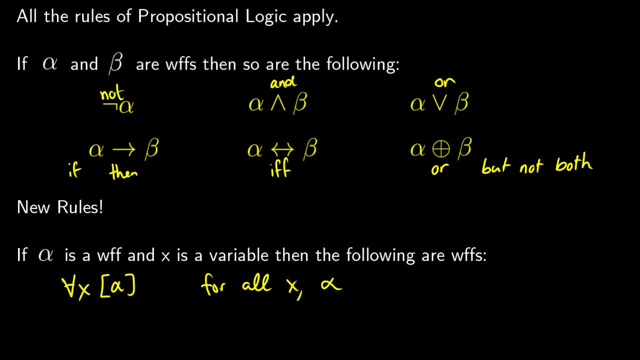 When we talk about sentence translations and meaning. We can also do it with the existential x. 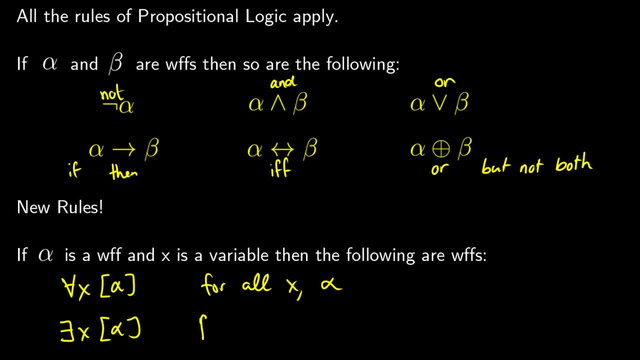 So there exists an x alpha. So we could write for some x alpha. 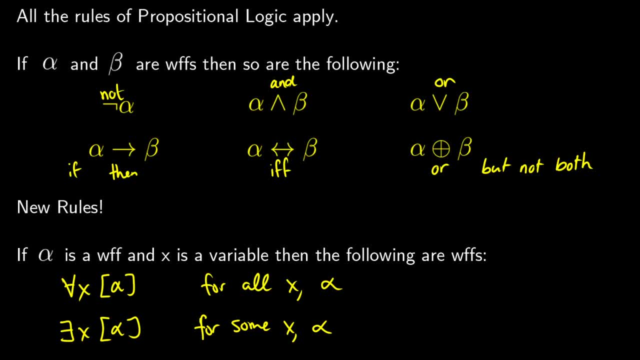 So again, don't worry too much about the meanings right now, this is just how we can make a well-formed formula. We'll talk about meanings in a future video. 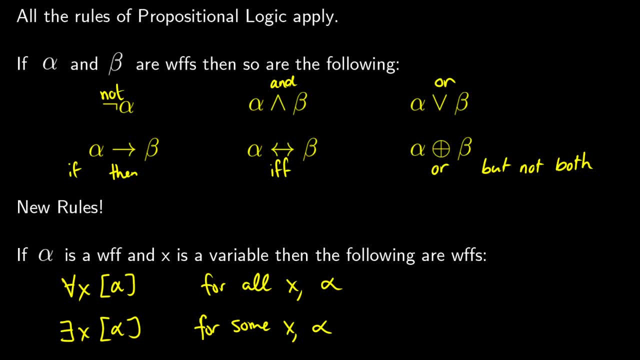 So we did some trees in the propositional logic section, but for example, if you have say for all x alpha, we can split this into two components. 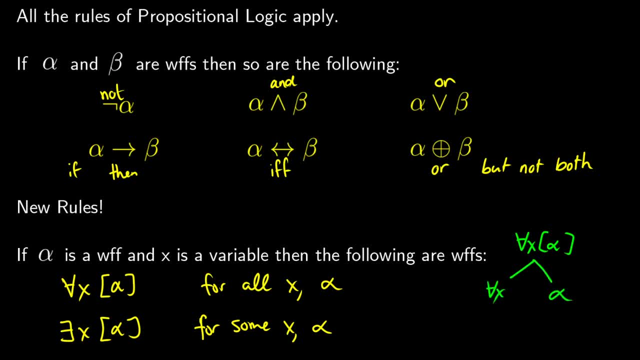 We can split this into for all x, and we can split it into alpha. 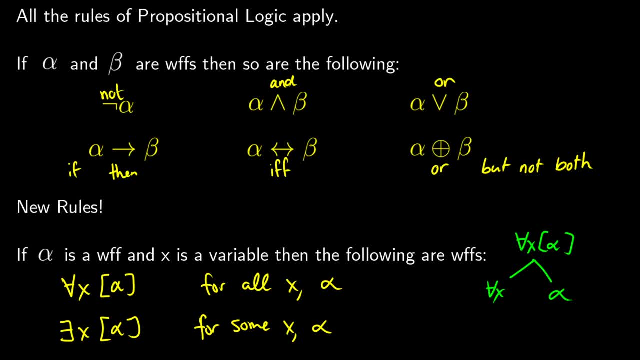 So that would be how we do a little tree for that, but we're not going to really focus on that in this section, since the syntactic structure of everything else should be straightforward at this point. 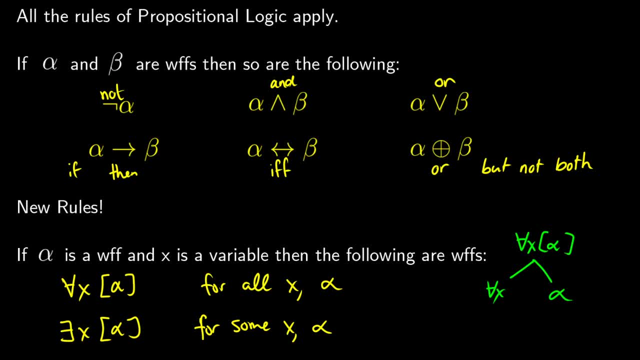 So I just want to say, it can really be any variable, in this position. So we didn't have to choose x, we could use y, z, or so on. 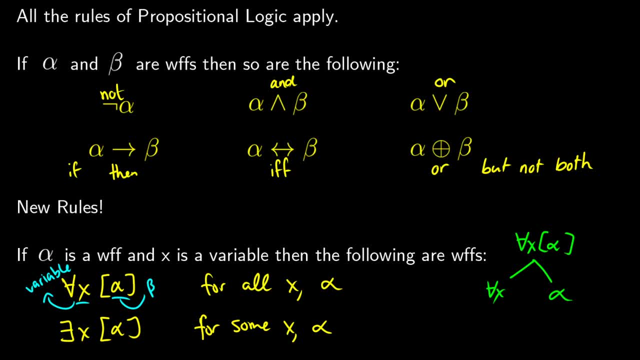 And we could also use any Greek letter at all. So this could be beta, gamma, or any other well-formed formula. 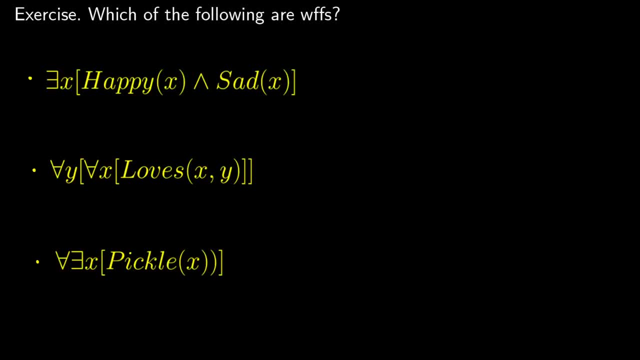 But we'll see what this is like as we go along. So just to finish off this quick video, let's ask ourselves, are the following formulas here well-formed or not? 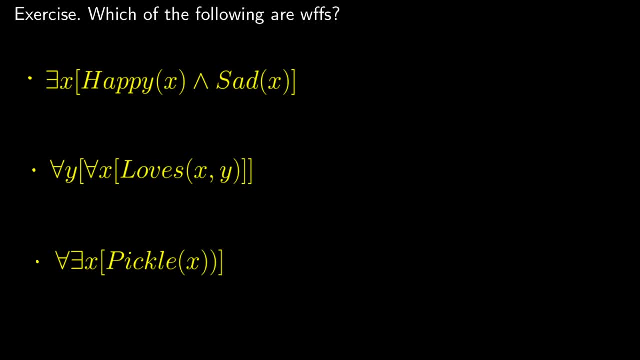 So what we're checking to see is, if we've constructed these formulas in a way that is appropriate. 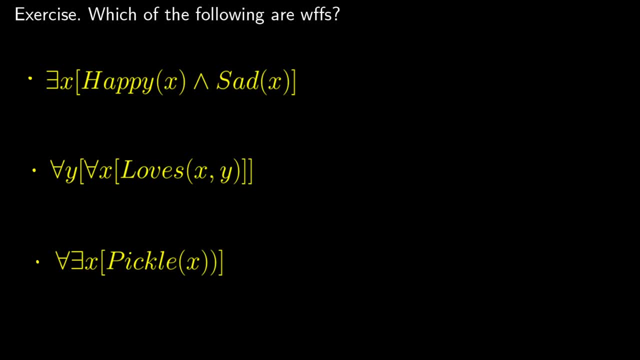 So the first thing to remember is that predicates combine with terms. So for instance, we have this predicate happy, and you can see I'm using full words here so we can understand what this means a little bit better, just to give ourselves something concrete. And this combines with a variable x. So happy x could be something like x is happy. Okay. So that's good. 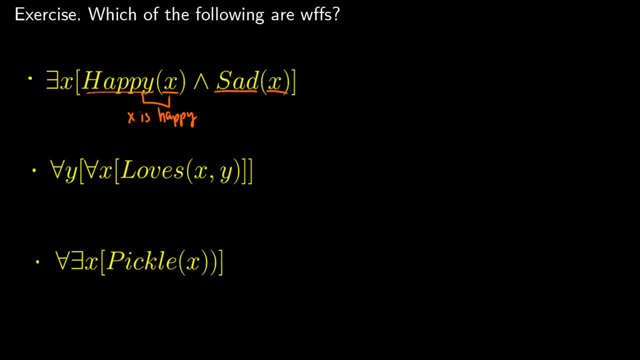 We have a predicate sad combined with some amount of terms. So this could be read as x is sad. So these are two well-formed formulas. This is like alpha. This is like beta. And we're combining them with and. So we have an and in the middle here. So really what this internal part is saying 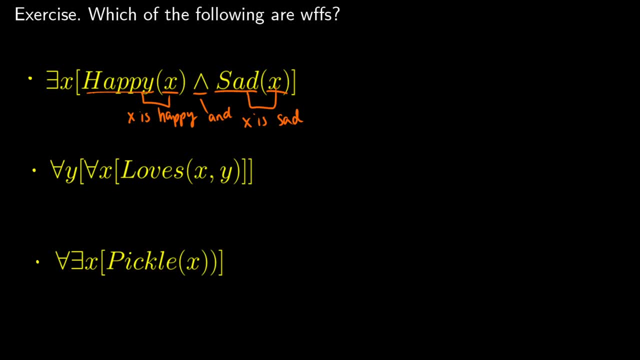 is that x is happy and x is sad. So this entire thing we can treat as one well-formed formula. 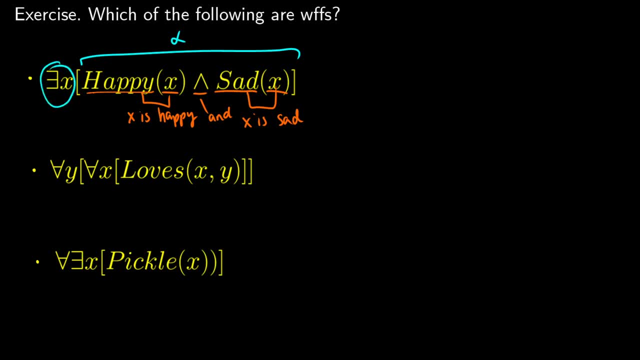 Now on the outside, we attach an existential marker with it. So existential with the variable x, and this associates with alpha. So this is saying there is some x such that the following is true. 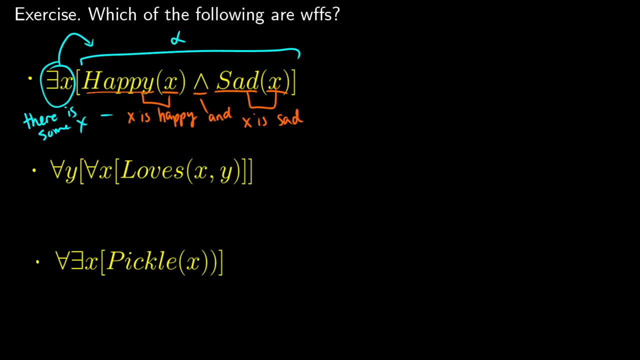 So there is some x such that x is happy and x is sad. So ignoring the meaning, this is a well-formed formula. This is a woof. 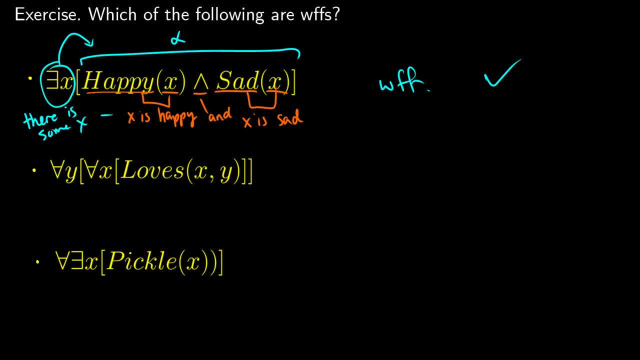 Okay. Let's take a look at the next one. So this one has two quantifiers on it. But let's start with the inside. We have a predicate loves. 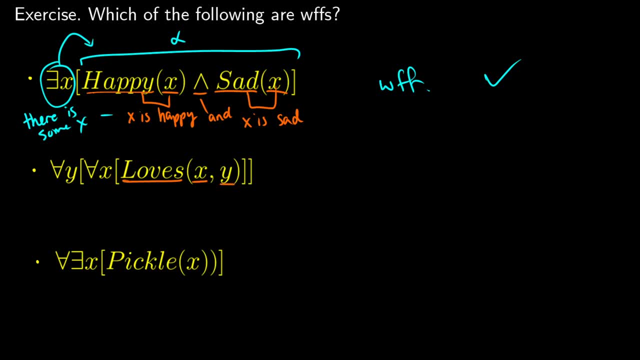 And this is going to take two terms. So x and y. And this is fine. 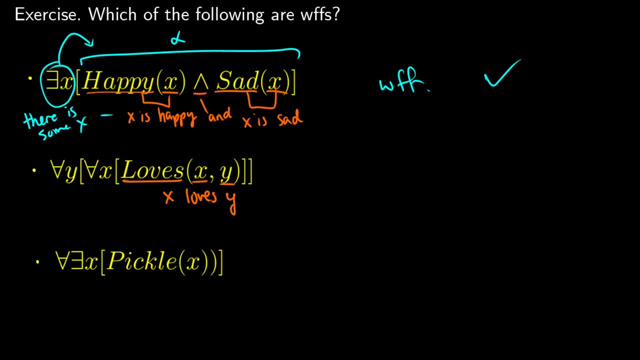 So this could mean something like x loves y. We don't know who x and y are. That's okay. 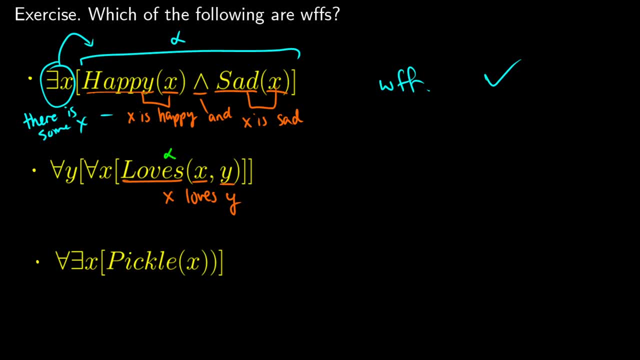 So we can treat this as a well-formed formula alpha. Now we can combine the universal x with this. 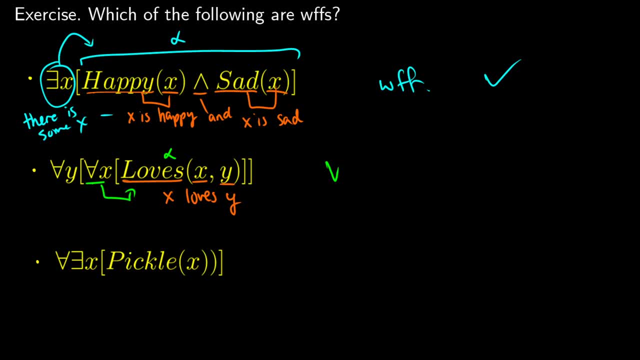 So basically what we're looking at here is just abbreviating everything for simplicity. We have something like for all x alpha. And yeah, that's good. 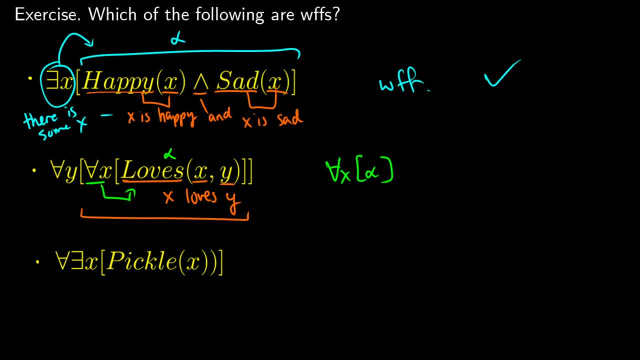 So that is well-formed, which means we could treat this whole thing like a new alpha. And then that means that we have for all y alpha or beta, whatever we want to choose. So we're connecting for all y with another well-formed formulas. So yes, everything here is good. 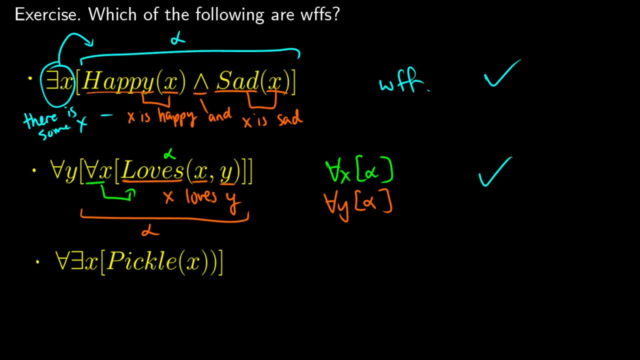 This is a woof. Now the last one. Is this well-formed? Well, I mean, if I'm giving you two good ones, the last one is probably going to be bad because this is a tutorial video on how to understand this stuff and put this stuff together. So pickle x. This is fine. 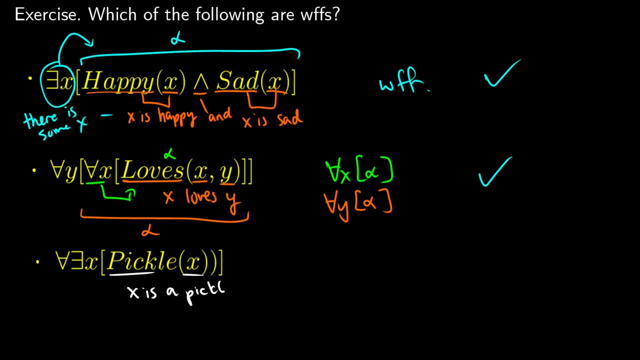 This is like saying x is a pickle. We're giving it the property of being a pickle. 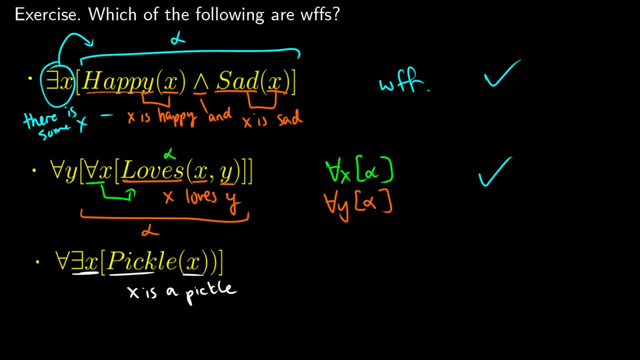 And now we combine it with this existential x. So we've seen this before. 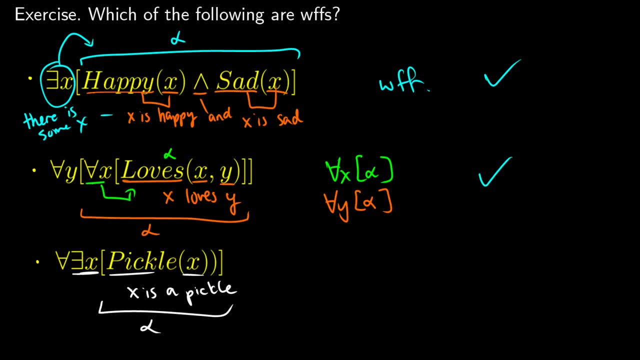 If we treat this as a well-formed formula alpha, we get exists and x alpha. And that's good. 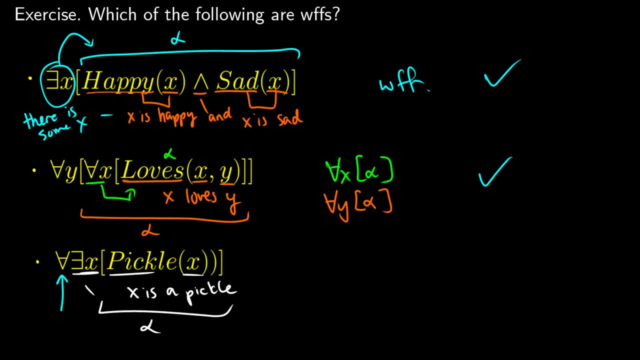 What's problematic is this for all. Because this for all doesn't have a variable beside it. 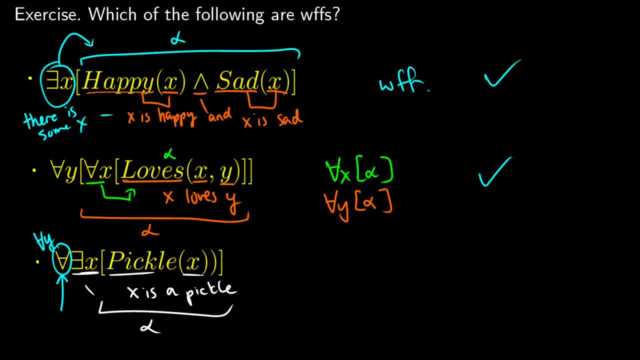 It needs to have a variable, like for all y or for all z or something. But because we just have for all exists and x, this is not going to be okay. So we can put an x through that, and we can say okay, because of that, no, this is not a well-formed formula because it doesn't follow our rules. 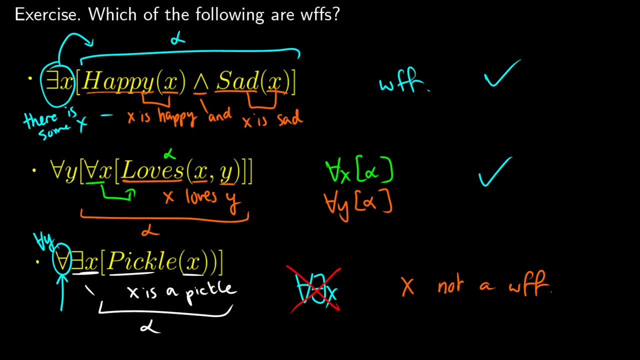 If we ever have a quantifier like for all or exists, we need to have a variable immediately after that. 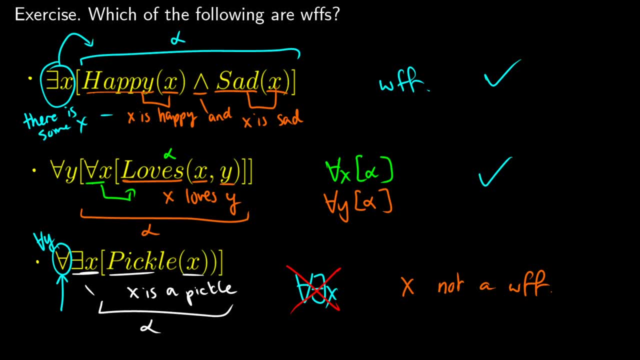 So you might be thinking at first, and if I just sort of clear everything that's on the screen here, 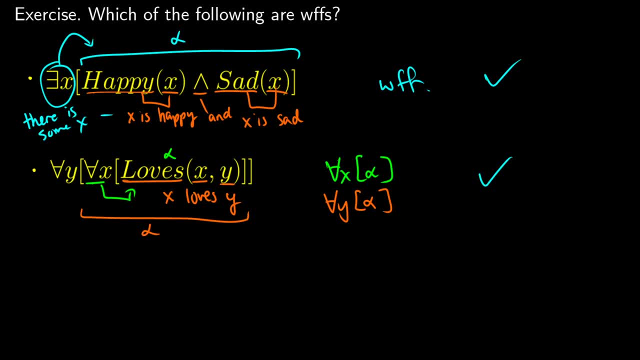 at least for this example, well, that just took the whole thing out. Never mind. We don't want that to happen. 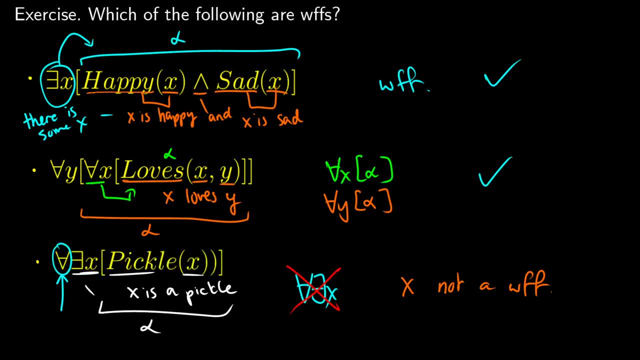 If we just take a look at this for all exists and x, you might be thinking initially, this is just shorthand for all x exists and x, 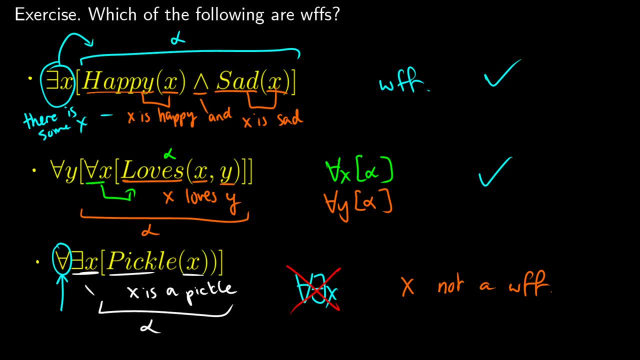 but that's not true. We need to have a variable after it. 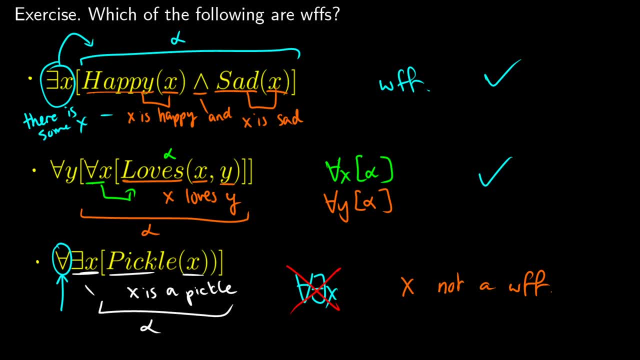 So this is a nice quick video on how to identify well-formed formulas in predicate logic and why we need to use predicate logic. 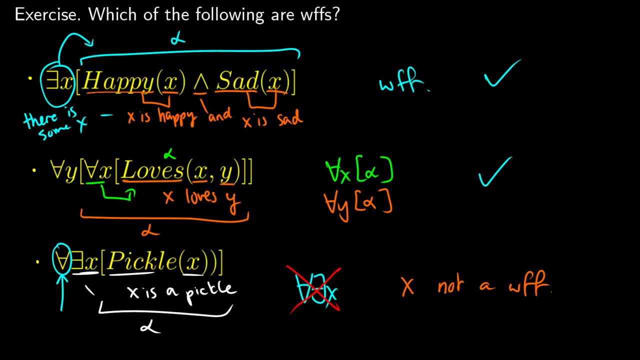 If you have any questions or concerns, I'm sure somebody in the comments will answer you below, or maybe I'll be able to get to you. So thanks for watching. 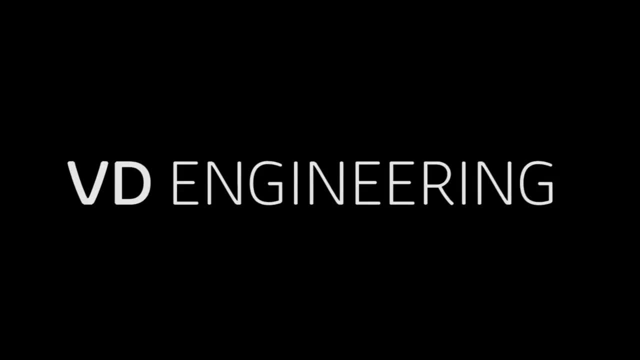 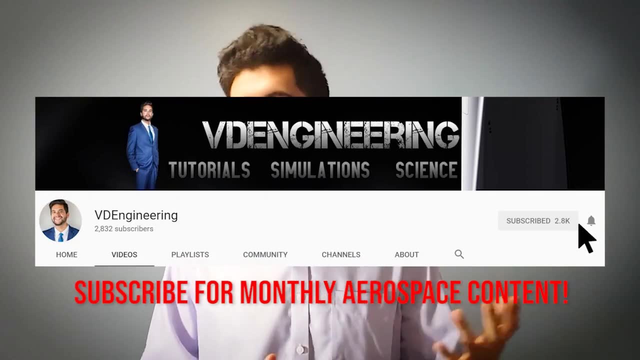 Hey guys, what's up? Vin here from VD Engineering and in this video I'll be showing you guys how you can use MATLAB, Simulink and FlightGear to build a simulation of a spacecraft attitude control system.